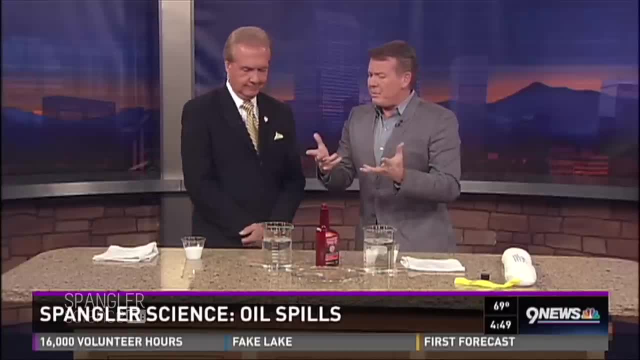 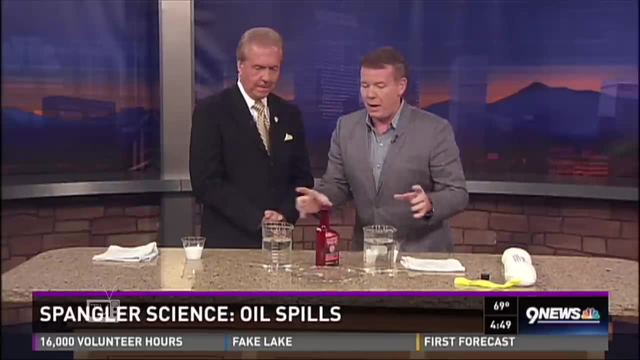 I know I love it. We love it when you're live from the ship. So and we're going to talk about everybody always asks about the oil spill. That's one of the first things they ask the rangers: Have we completely recovered from the Exxon Valdez? I wanted to show you some of the technology behind it. 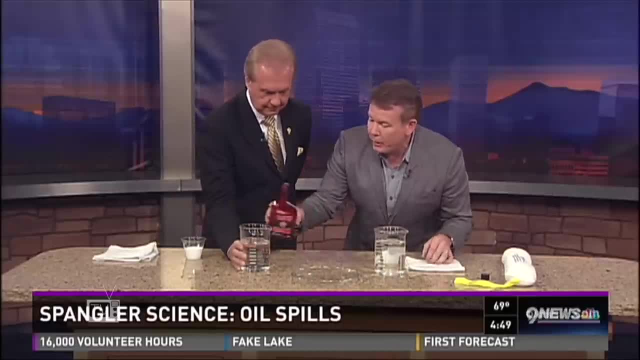 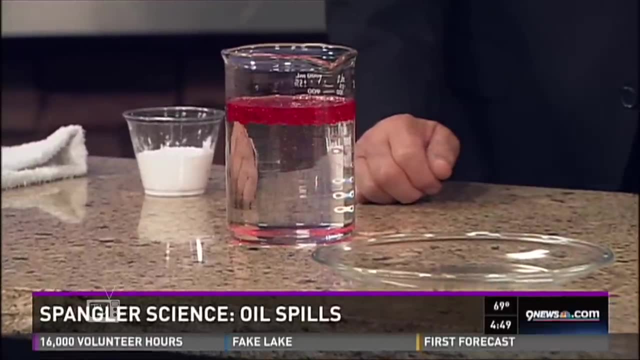 You have a glass of A container of water. I have a container of water. We're going to use something that's similar to that same crude oil that you would see before. This is synthetic. This is a material called Marvel Mystery Oil. We use it for the demonstration because it's red and it looks great. 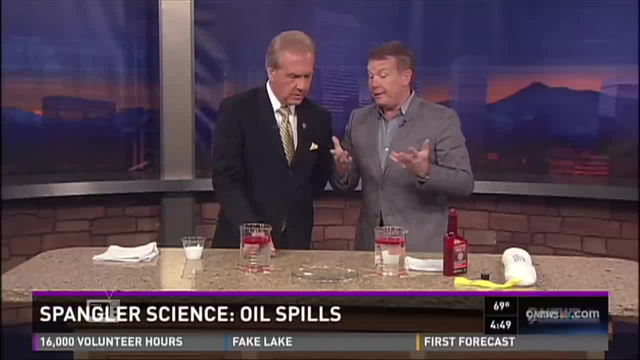 Does it float to the top like that in the ocean as well? Is that what happens? It does yep. So thank goodness, because as soon as it goes to the bottom, that's when the danger really sets in. Oh, I see. 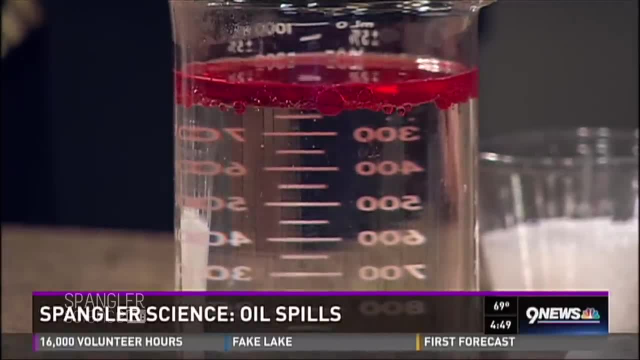 Because that's when you can't control it. So going in and putting detergent on the oil to try to clean it up makes it disappear in the public eye And the public's happy about it because it's gone, but it's not really gone. 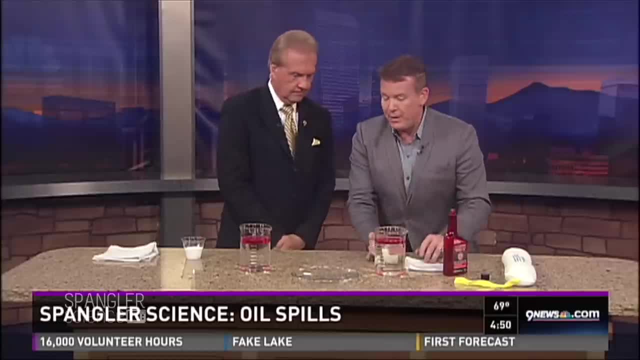 So everybody says that's maybe one of the worst things you could do. I see This is a polymer. Take a look at this. I'll sprinkle some on the table here. It's kind of coarse. You can put your fingers in it. It's perfectly safe. 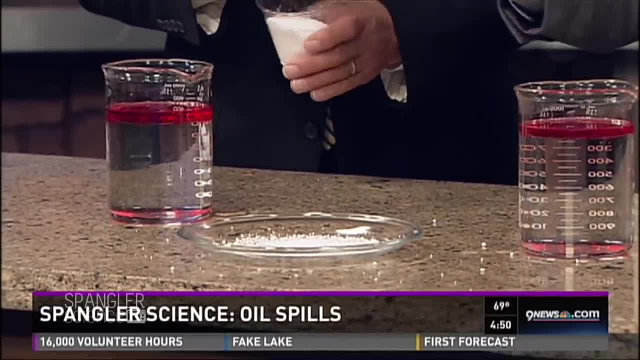 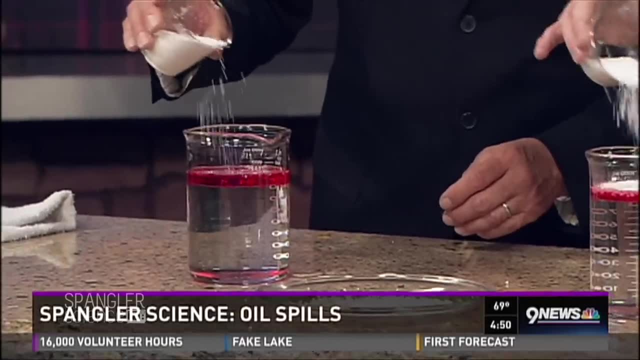 This particular material here will grab onto the oil. So here's what I want you to do is I want you to slowly sprinkle it in yours, And what you're going to see is not absorption, but adsorption. It just means that it hooks on the outside. It's AD instead of AB. 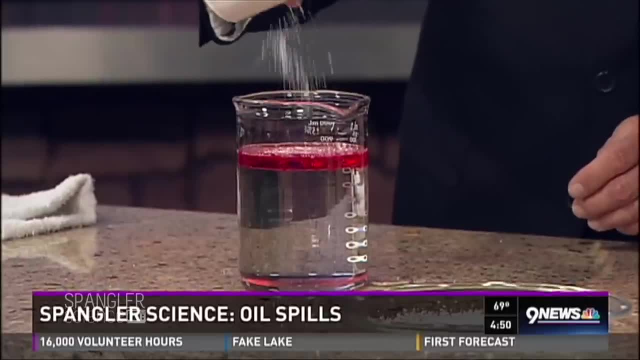 Oh, I see, So it collects it. Can you take a look at it? It does collect it Kind of in a one-to-one ratio. Do they do this, They do this. So go ahead and keep on going, More, more, more. 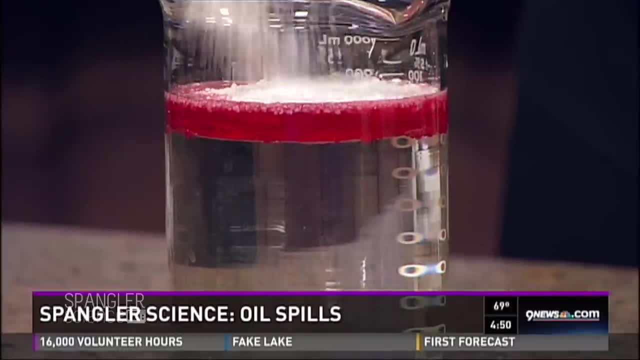 You can even do more. There you go. So what's going to happen is this: You can see that it's starting to – yeah, there you go. And so, as we move this whole thing around like this, you can see that it starts to form this layer. 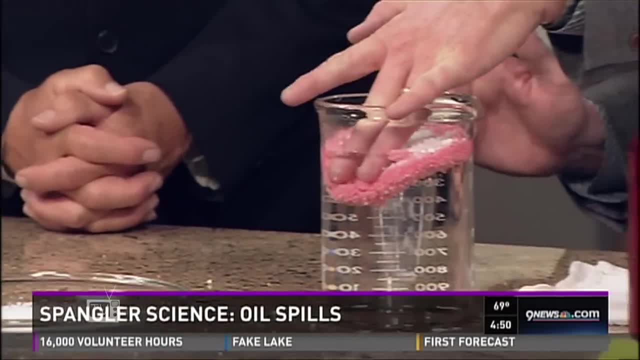 Take a look at this. I'm going to push down. Would you look at that? Oh, for heaven's sake, It's like a little cake, Like a little cake that's there, A polymer cake. So, believe it or not, they can use this kind of technology. 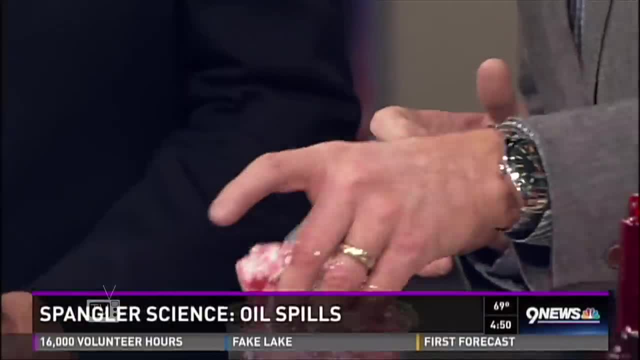 Gee whiz, Look at this- to be able to remove the oil And take it right out of the water. So on the latest spills- Not in Alaska, but the latest spill that was happening in the Gulf Right. They used these in film. 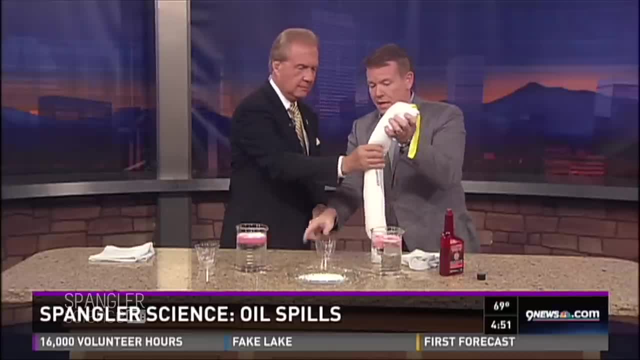 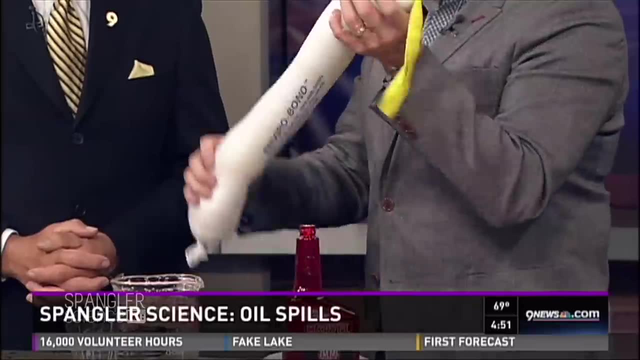 Booms You got it Is that the booms you were reporting? And they put the polymer inside here and then would set it down so when the oil would come and contact it. The problem is there was so much oil they couldn't pick these up, haul them away fast enough to put the new ones down. 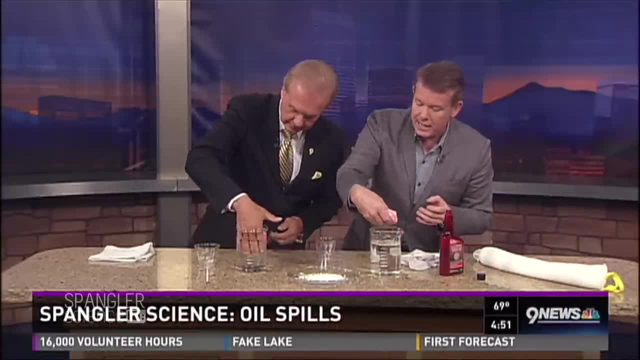 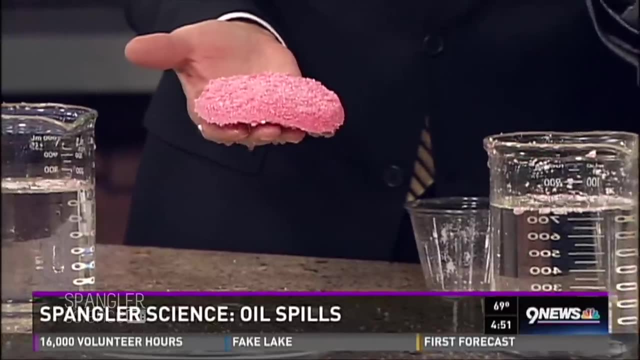 But here, reach inside and see if you've got it. Look at this: It becomes a solid. And there it is. There is your solid. So there is technology. This can go on the birds' feathers and the wings. They can use this to clean up on the beaches. 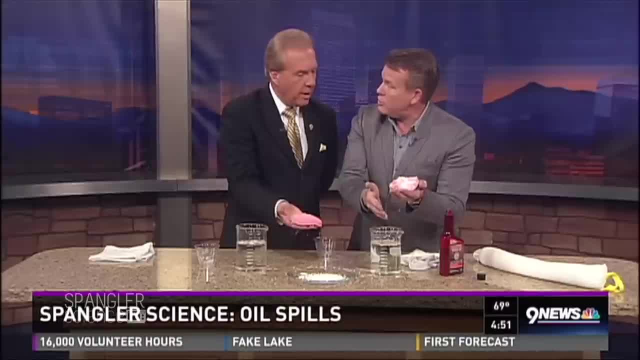 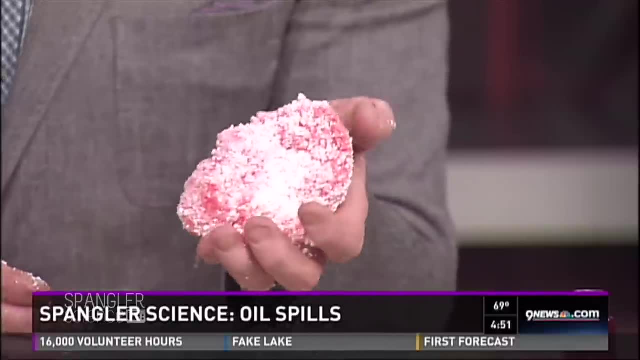 And it's amazing, This is a polymer that grabs onto that oil, So the technology is great. Is this the same polymer in baby diapers that we use all the time? No, That's an absorbent polymer, But this is specifically for oil, which is fascinating. 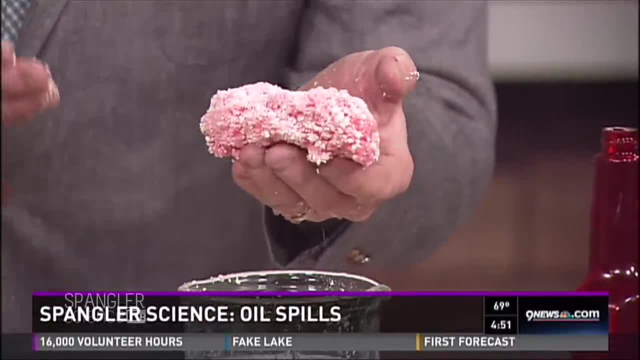 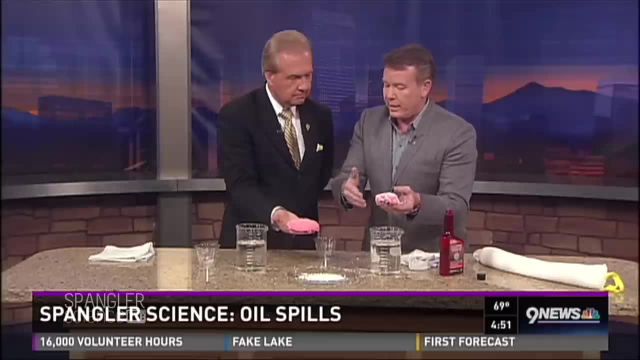 And the greatest part is the guy who invented this. well, the bad thing is he passed away before they ever saw it used in this type of commercial application, Because the government had some regulations about sprinkling this powder in the open seas. They want you to contain it like this. 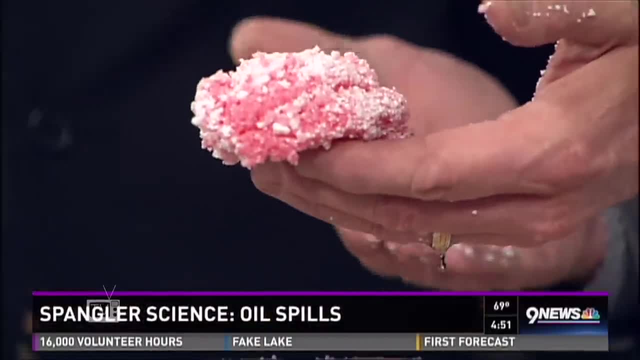 But you can see how effective this is. That is amazing. So it's been an activist project for kids all over the country to say this is what we can use. Unfortunately, when those spills happen, you can actually burn this and there's a BTU rating on it. 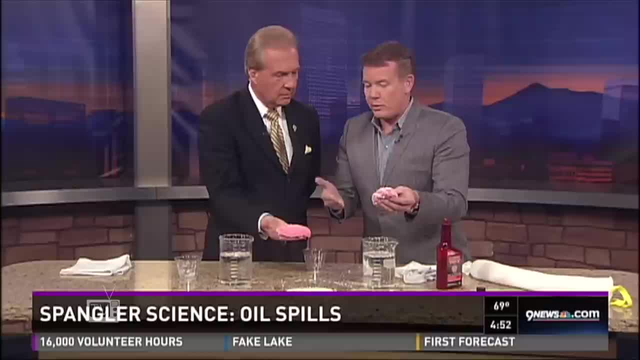 Really And you can extract some of the energy. No kidding. So the guy was absolutely amazing. It's a great inspirational story for kids to understand that the science is right there, at their fingertips- Another way to save our oceans. You got it. 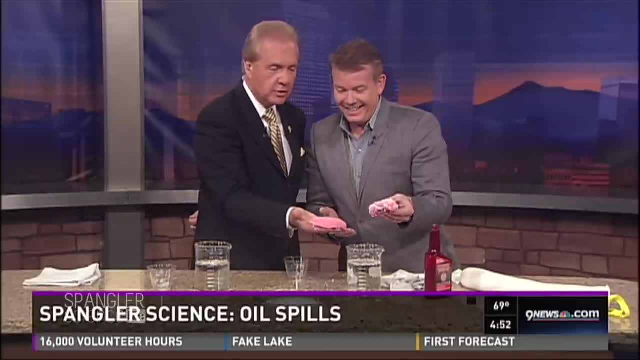 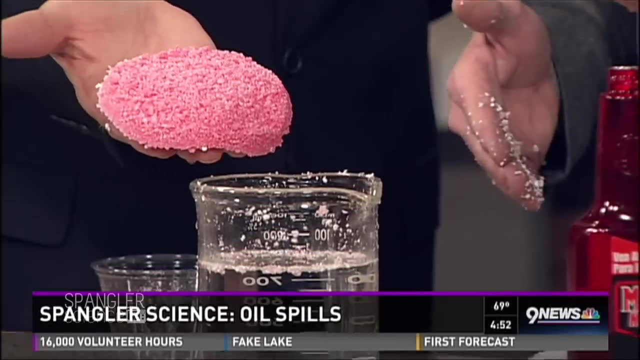 Can I point to something else that I've learned here? Yes, Mine, Can you see these cherries? Put mine next to Steve's. Mine looks much nicer than yours does, And you are. you've done well As a scientist. I just want to say this rarely happens for me. 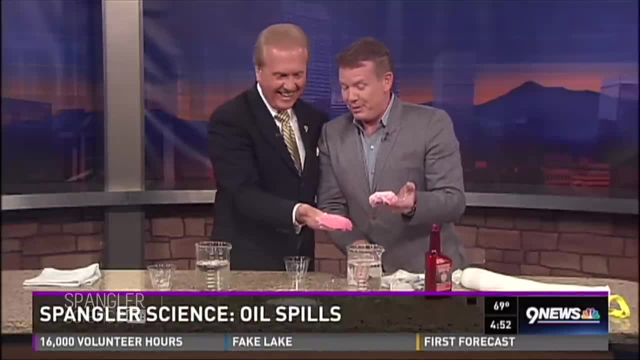 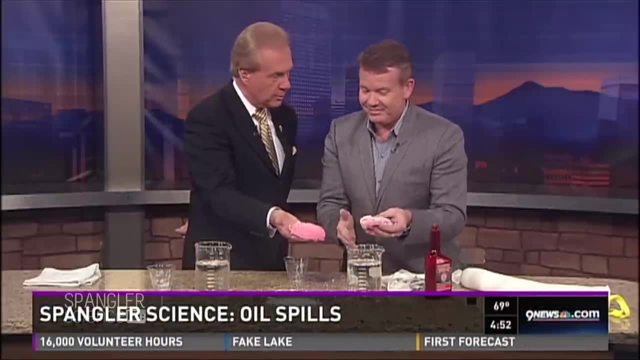 I actually have. It's so much better. So you get to take this home now and put it under your pillow. I think that's amazing. It will be there in the morning, but you get to take it home. You know, Kim and I were just. we report on this all the time and we see the booms go into the water. 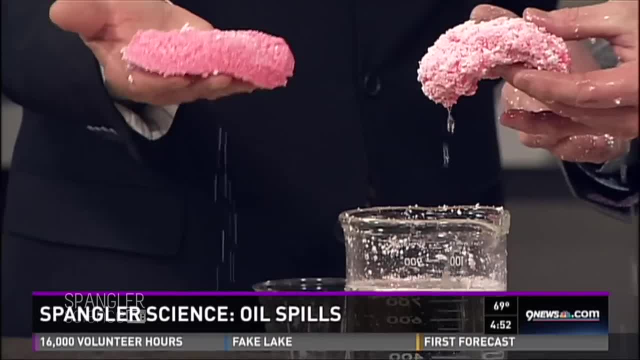 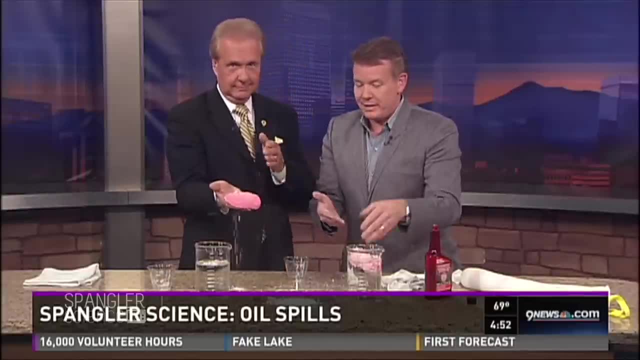 You got it And we watch this And you know, and a lot of the oil hits the beach before they get this down And that's always really cleaning the sand and the rock. But it is there and it's a guide, just like you and me, that would sit there and kind of come up with this wonderful idea. 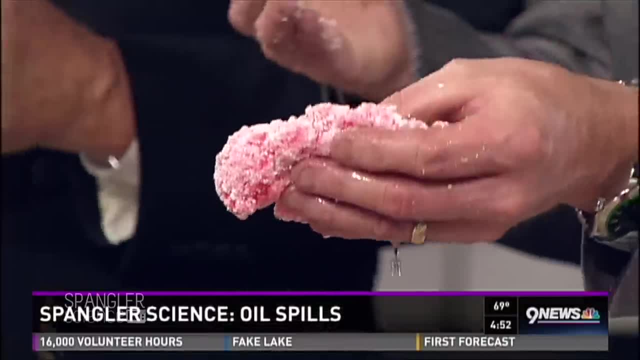 What a great way to do it. So we're going to report live all next week, Okay. You're going to follow us on Facebook at Steve Spangler, Okay, And we'll share what these hundred teachers are doing. We're looking forward to it. Thanks, Science Guy.